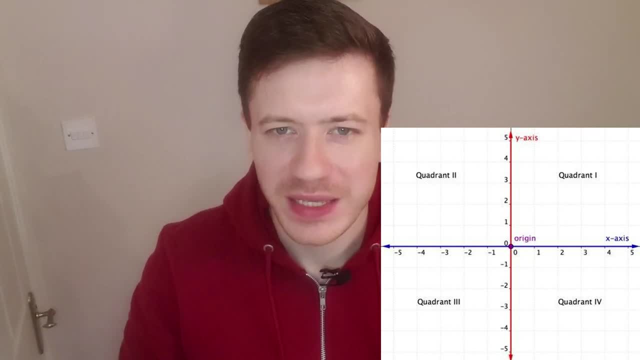 three and four beneath quadrant one. Many students- and I used to believe this before I learnt- thought that quadrant four was in the bottom left in the negative negative axis, but that's not actually true. It goes quadrant one in the top right and then. 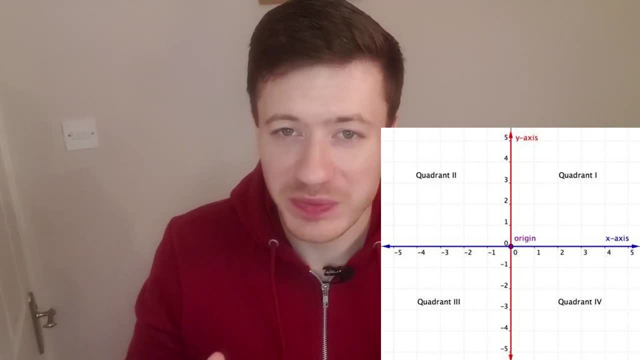 clockwise quadrant two, three and four. I'm surprised by how many students don't actually know that, so that's definitely useful knowledge. if you didn't, Next, you need to know that the y-axis is the vertical line and the x-axis is the horizontal line. I'm sure many of you knew that. 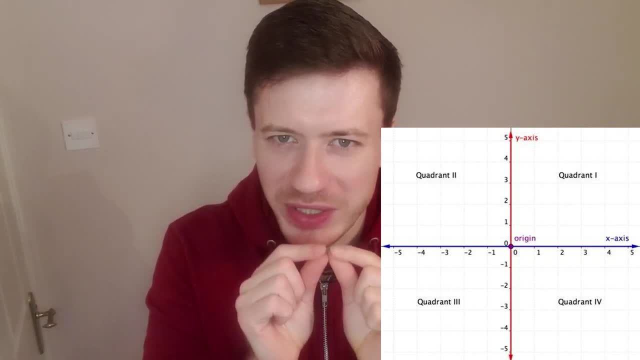 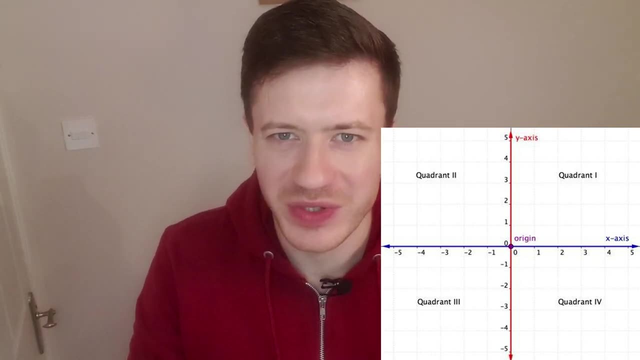 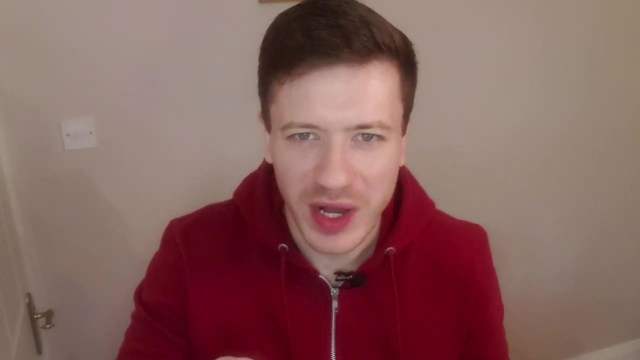 already? Did you also know that the origin is that point right in the middle, zero, zero, where the x-axis and y-axis meet? You probably did know that, so I'm going to move on to the next topic, which is finding the line. You might have heard of this famous equation y equals mx plus b. that you can see on: 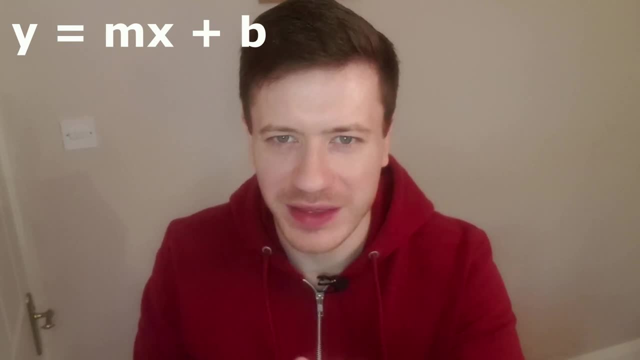 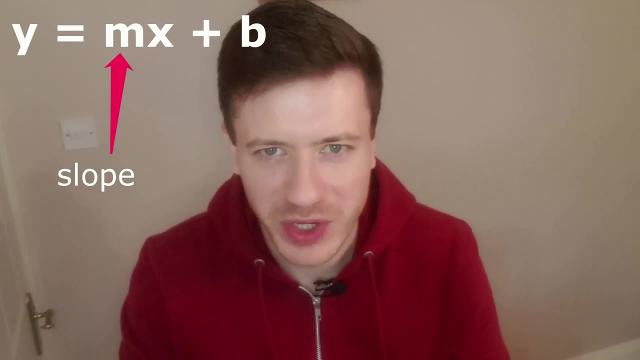 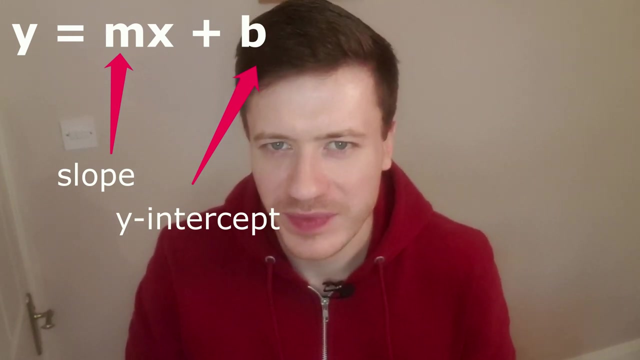 screen. But what do the letters mean specifically, the m and the b? The m is the slope of the line, that's the gradient some people know it as, and the b is the y-intercept of the line where it crosses the y-axis. Now, many people know that, but they're actually a bit foggy on how to calculate. 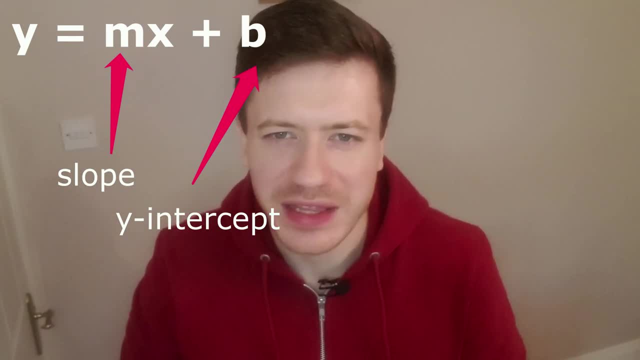 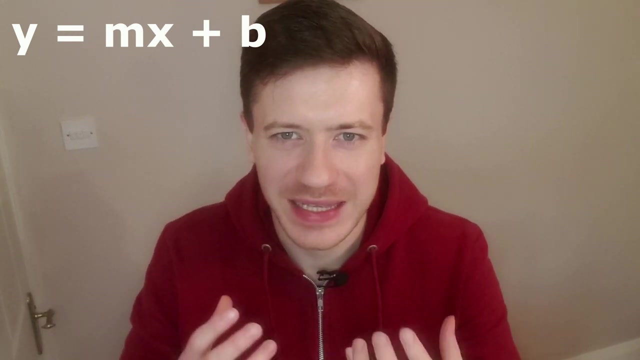 the b, and if I gave them two coordinates, they wouldn't really be able to give me the equation of the line. in that form, y equals mx plus b. So that is what our first question is about, and I want to add in at this point that all the questions we're going to do today are phrased exactly as they. 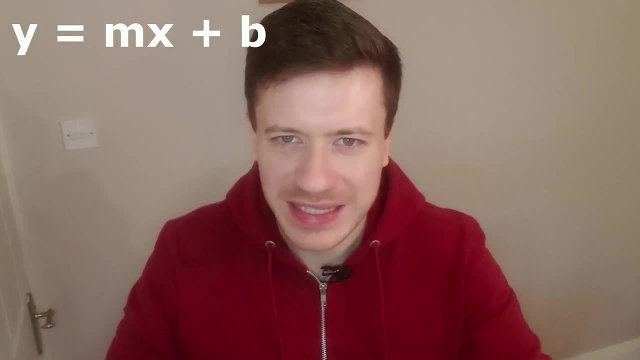 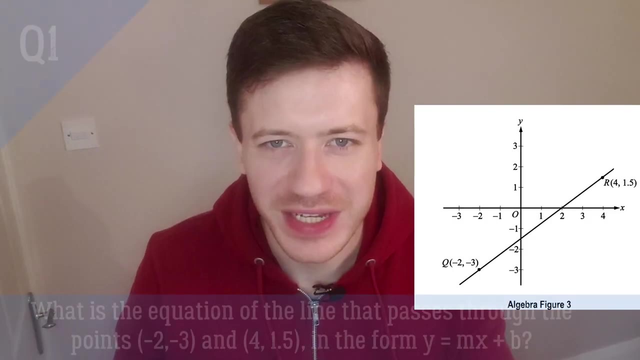 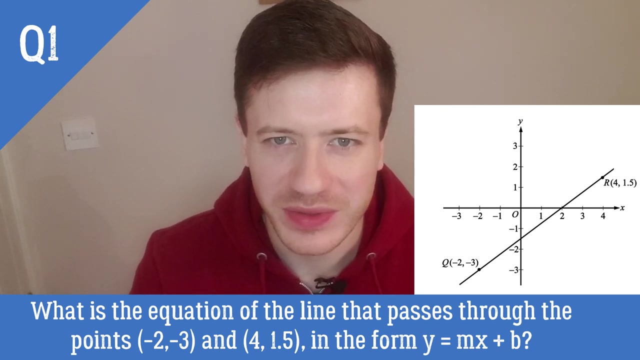 might be. in the real GRE or GMAT exams. They're tested in a very similar way. In fact, two of the questions I'm going to use are from the actual official ETS math review. Here is the first official question. The line you can see on screen goes through the points minus 2, minus 3 and 4- 1.5, and I'm going 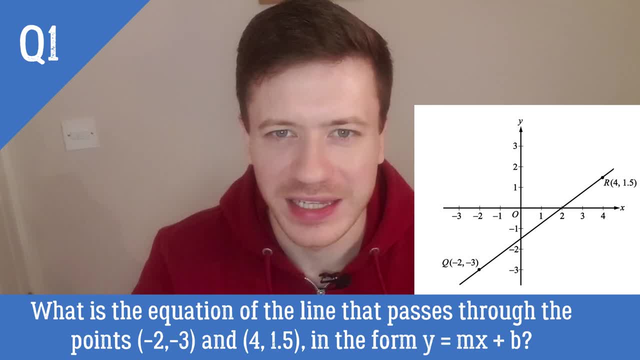 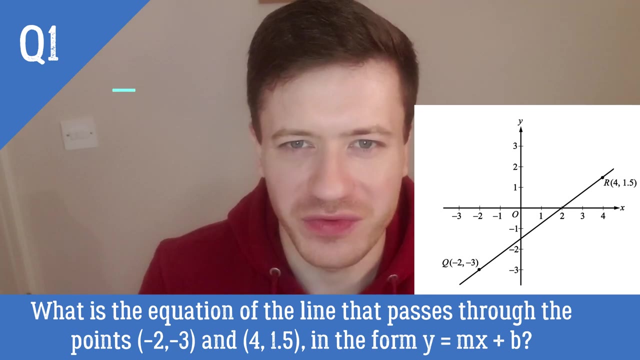 to ask you what is the equation of that line? in the form, y equals mx plus b. If you think you know how to do it already, you can have a go. and for everyone else, I'm going to teach you how to find that m and how to find that b. To find the slope, I'm first going to get you to think of it as the 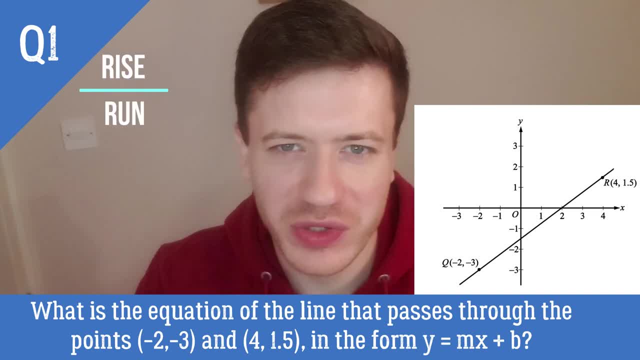 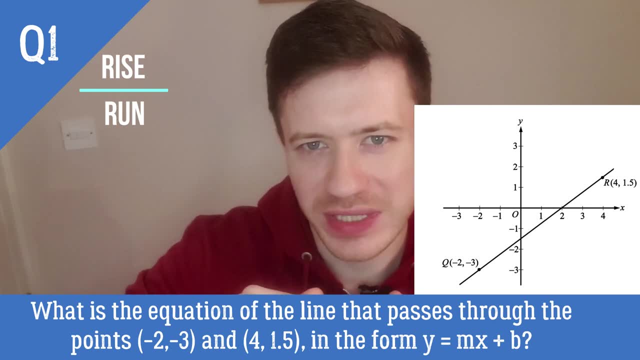 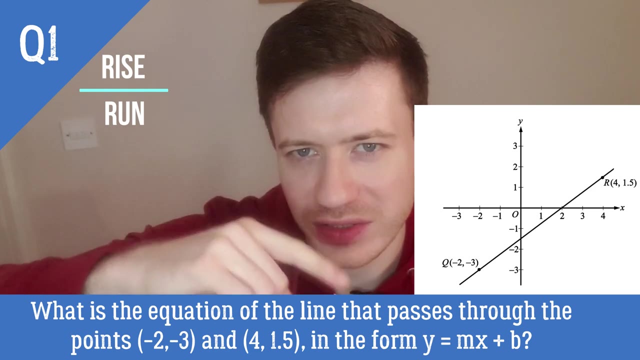 rise over the run, and later I'm going to give you the formula. So you have two approaches to think about with the slope. First, the rise over run approach. That's where you consider, by picking one of the coordinates, how far has it risen in the vertical or y direction to get to the next. 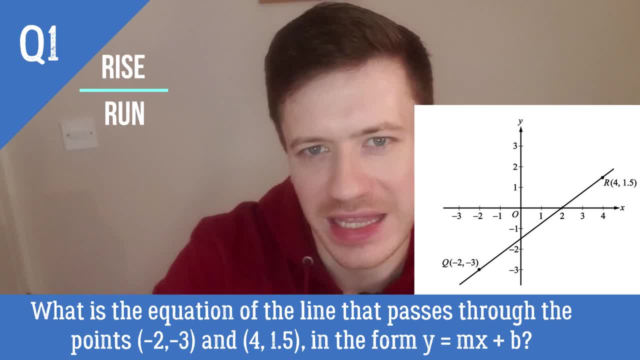 coordinate and how far has it run. in the x coordinate direction, the horizontal direction, You find out how much it's risen and then divide that by how much it's run, and then you would have your slope. We're going to use that approach first. 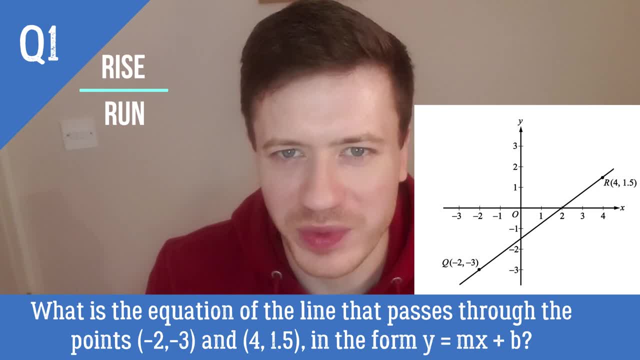 with these coordinates and then afterwards we're going to use the formulaic approach. Before we get started, remember that the coordinates on the left are the x coordinates, the horizontal coordinates, and the numbers on the right are the y coordinates, the vertical coordinates. So let's take our coordinate on the left minus 2, minus 3.. How far has that risen? 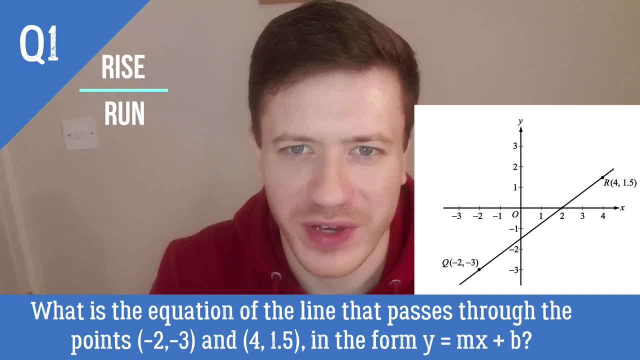 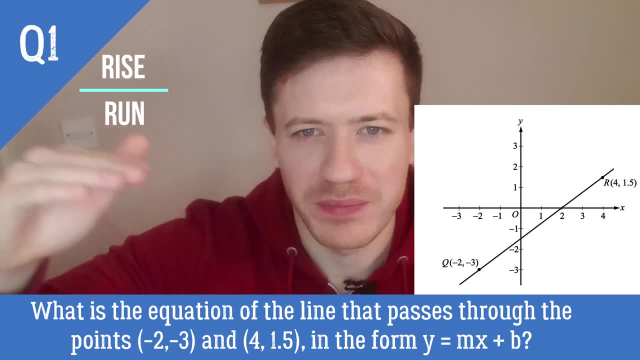 to reach the coordinate. So we're going to take our coordinate on the right for 1.5.. For this we need to look at the y coordinates. So we've gone from minus 3 to 1.5. That's a jump of 4.5.. To get from minus 3 to positive 1.5, we have 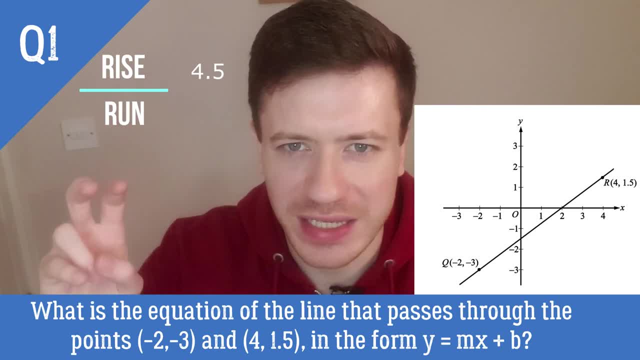 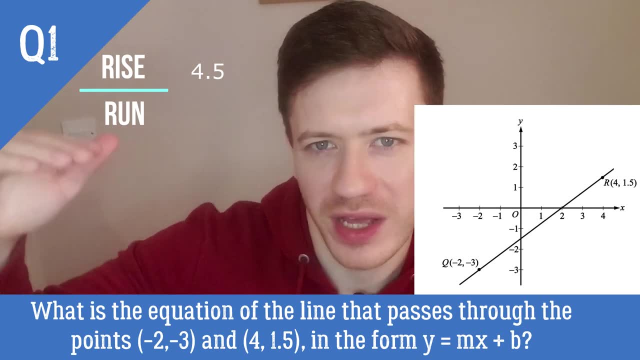 to rise by 4.5. So that's our rise on the top of the fraction. Of course, by the way, if we'd have gone down we would have written that as a negative number. but no, we've gone up by 4.5.. Now can you calculate our run? 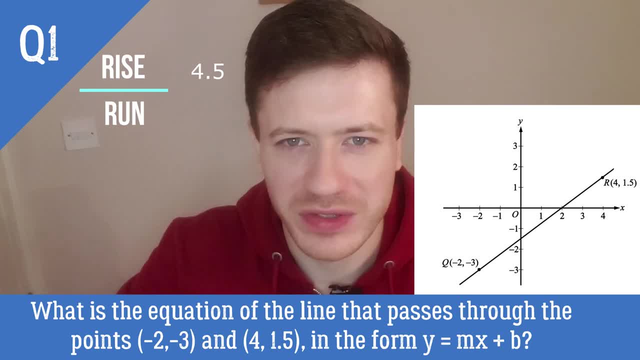 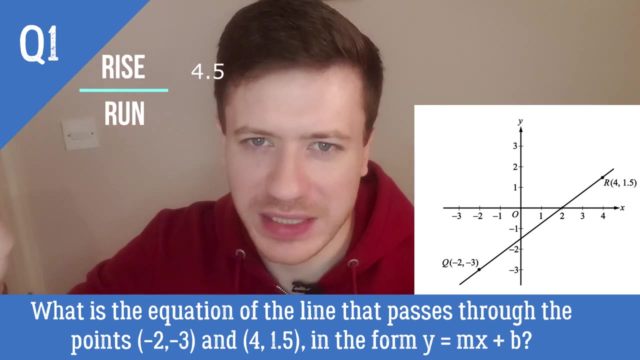 How far have we gone across in the horizontal or x direction between those two coordinates? You always must consider the same set of coordinates. You must start with one coordinate and go to the other one, not mix them up, not start with the other coordinate and go back to. 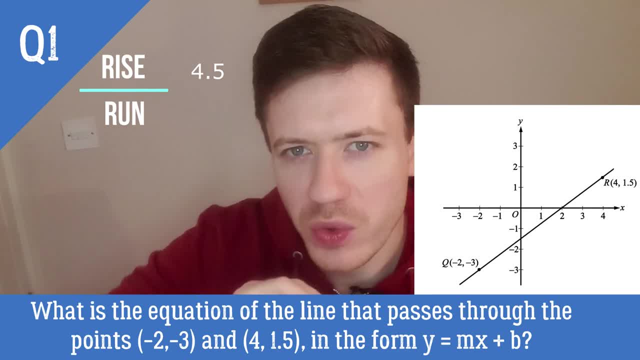 the first one. We're going to start with that coordinate on the left and always be focused on getting to the coordinate on the right. What's the run? Well, we've gone from minus 2 to positive 4.. So that is a run, I think, of 6.. From minus 2, x coordinate to an x coordinate of 4.. 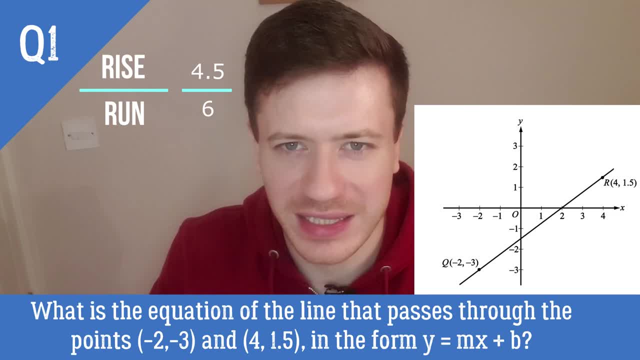 Minus 2 to 4, that's 6.. So our run is 6.. Our rise was 4.5 and our run is 6.. So we have the fraction, the slope, 4.5 over 6, which of course we can double to get rid of the decimals 9 over 12, and we can. 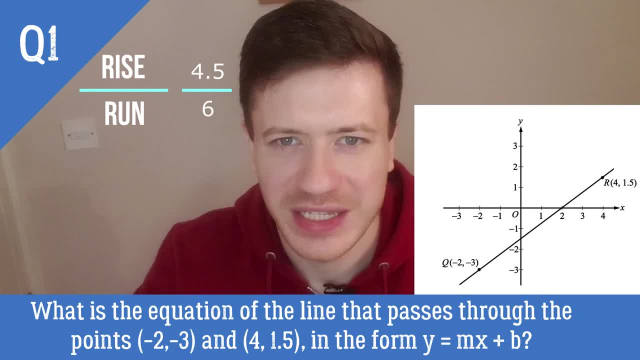 simplify that down to 3 over 4.. So 3 quarters is the slope of that line. Now, just quickly, for those of you who love formulas, we have the formula y2 minus y1 over x2 minus x1 to calculate the rise over the run. Essentially it's a formula. 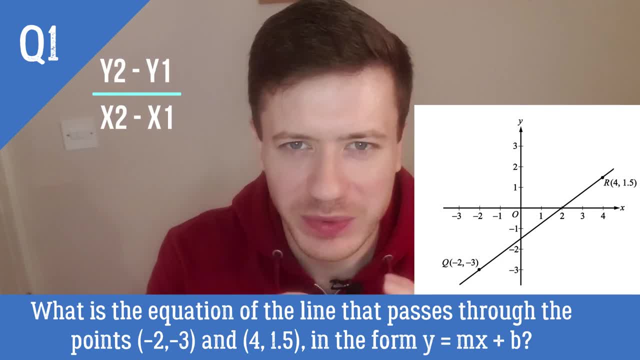 used to calculate the same thing we just worked out. You label one set of coordinates x1, y1, let's say that's the minus 2 minus 3, and you label the other set of coordinates x2, y2.. You can call that the coordinate on the right for 1.5.. Then we just churn it into the formula. 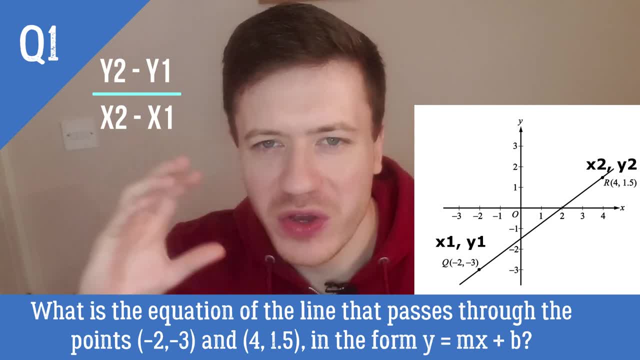 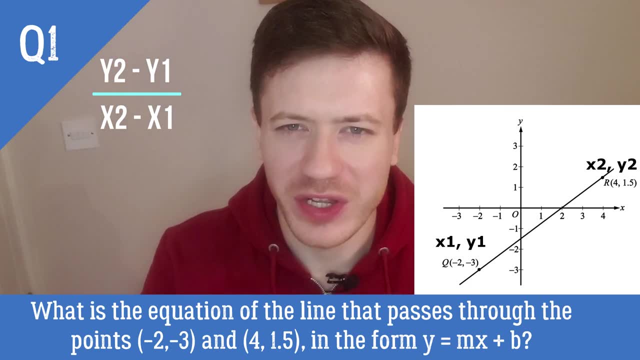 and out will pop the slope. So no kind of visualizing rise over run. you just chuck it into the formula and work it out. This is a better approach for those who are very confident with negatives, because a lot of negatives and double negatives tend to come up with this situation. 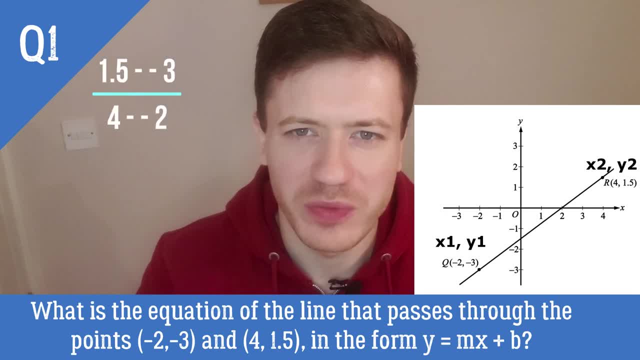 As we can see here, the y2 minus y1 would be 1.5 minus negative 3.. And the 2 negatives cancel out to give 1.5 plus 3, which is 4.5. And again with the run or the bottom side. 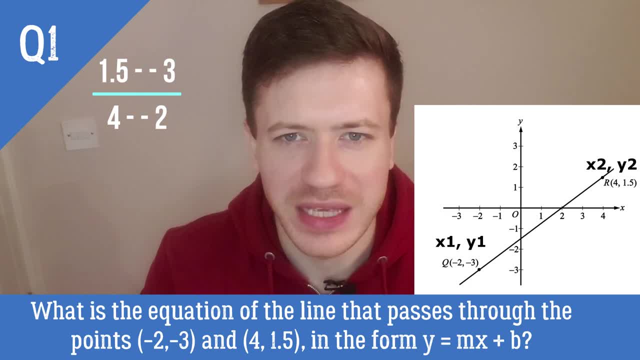 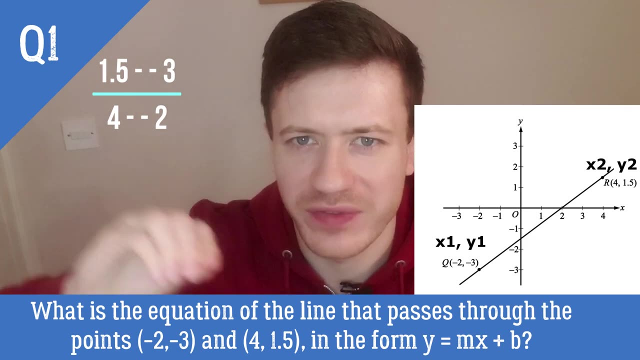 that's x2 minus x1. that would be 4 minus negative 2. And the 2 negatives cancel out to give us 6.. If you're confident with negatives, you can use that formulaic approach. if not, you can use the visualization approach. How far do we have to rise? 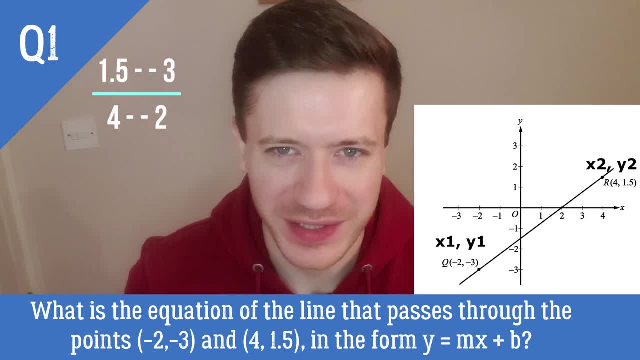 how far do we have to run? Either way, we have now worked out our our m. it's three quarters, so we can now insert that into our magical equation, and this is a key step that many students miss out. they have the slope and they're like: what do i do to work? 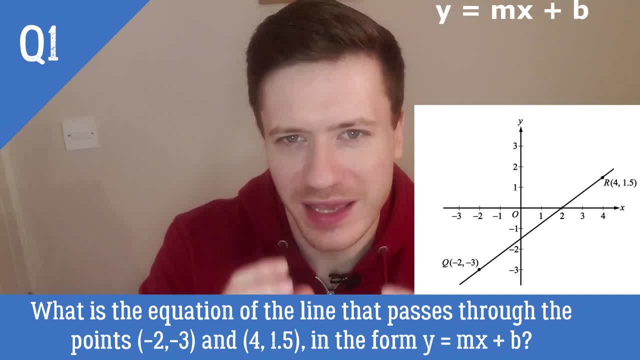 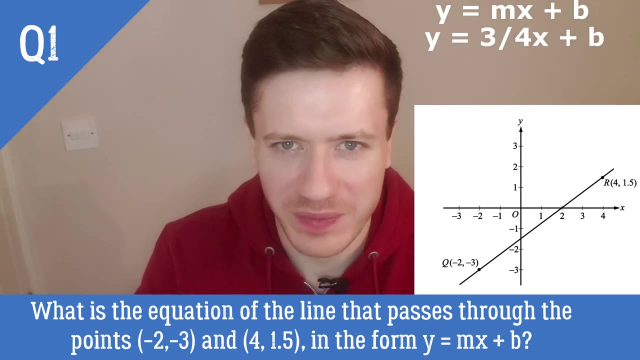 out the plus b. we're going to insert that slope. insert that m into that equation. y equals mx plus b. we would now have y equals three quarters x plus b. we're at the halfway stage. we've worked out the m, but we haven't worked out the b. that halfway stage is important. you've got to write. 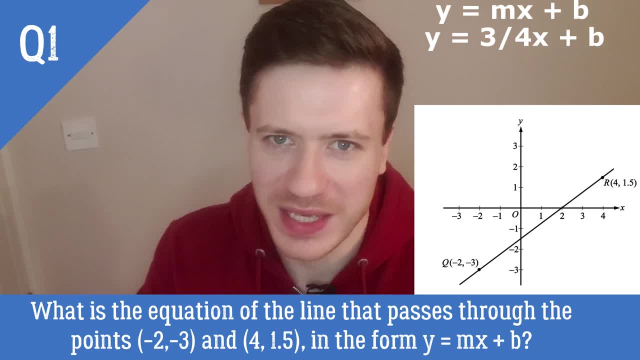 down that equation: y equals three quarters x plus b. how do we work out the y intercept if we don't have a visual graph to just observe where it is? this is the key step and this is why we wrote out the equation. we need to insert one of the points into our equation. many of you might think. 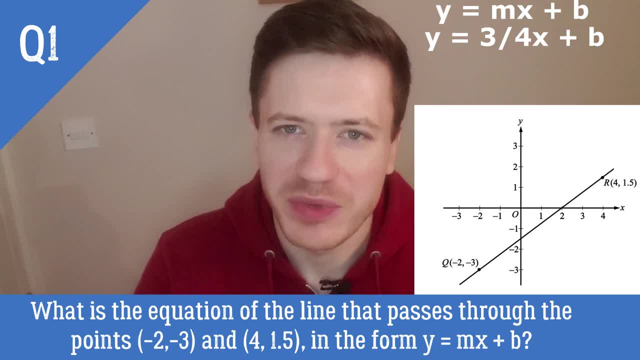 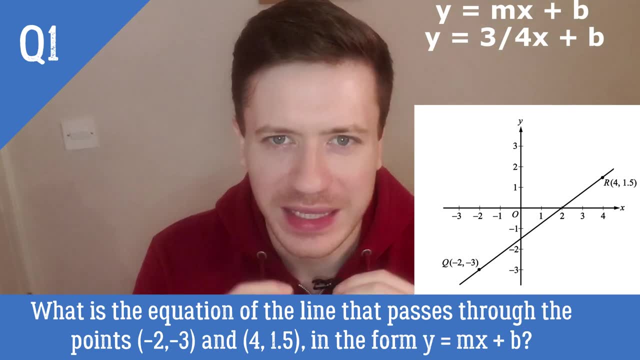 that the solution is to put x equals zero into that equation, but you'll find that it's not that. that will just tell you y equals b or something. it won't actually tell you what the plus b is. instead, we have to put both sets of one of the coordinates into the equation to work it. 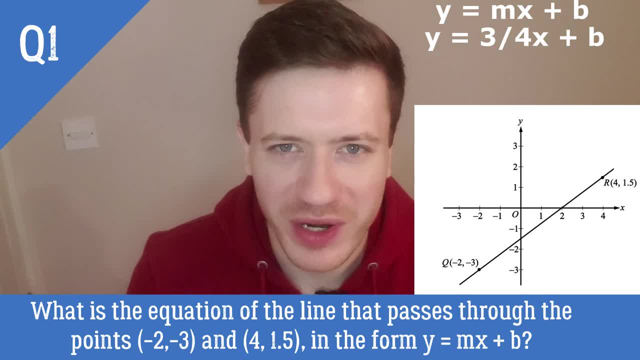 out. it doesn't actually matter which coordinate you pick, just pick one of them and insert both numbers into the equation. let's do that with the minus two and minus three. that's one of the coordinates on the line- and let's insert that into the equation. remember, our equation currently is y. 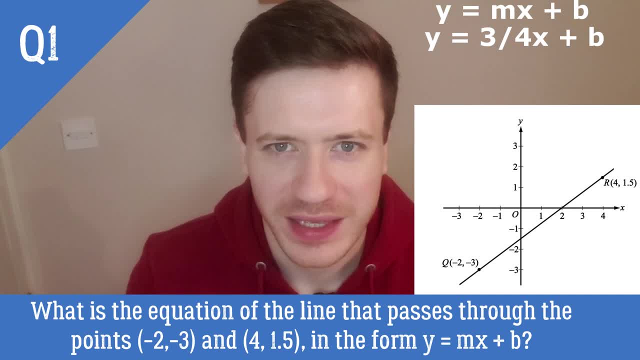 equals three quarters x plus b. with the coordinate minus two minus three, our x is going to be replaced with a minus two and our y is going to be replaced with a minus three. so we now should have- you can pause the video and do this yourself, or i can go through it: minus three equals three quarters times minus two. 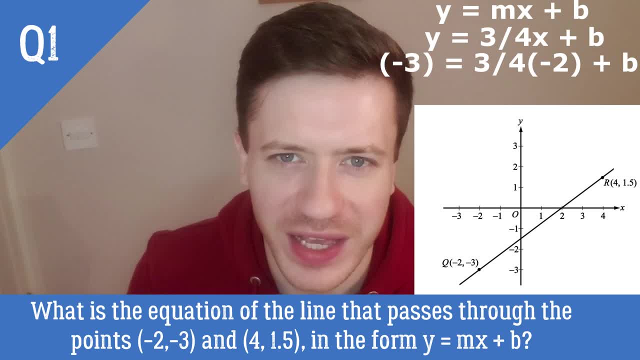 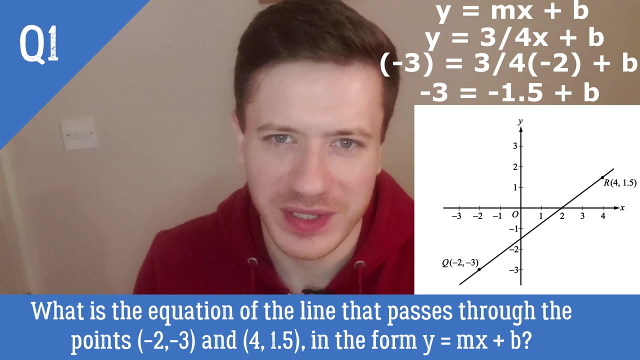 plus b, and that's how we find the plus b. working that out, you should have minus three equals minus six over four plus b. minus six over four becomes minus three over two or minus 1.5 plus b. so we have minus three equals minus 1.5 plus b. adding 1.5 to both sides, we would have 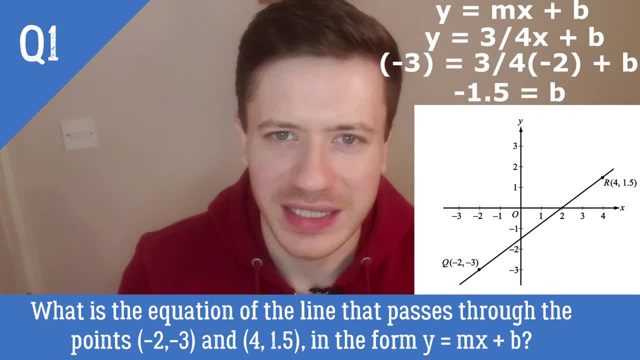 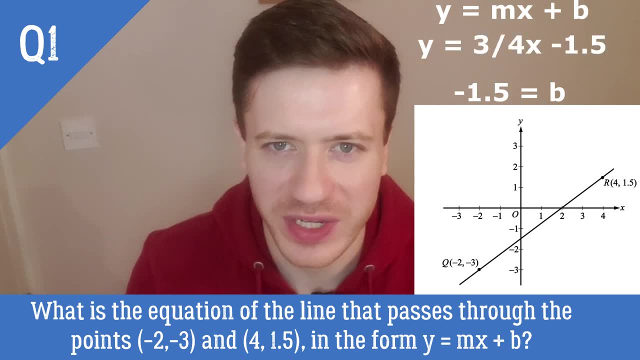 negative 1.5 left over on the one side equals b. so that's our b, that's our y intercept: negative 1.5 or negative 3 over 2.. of course you could tell that from the graph just by looking at it, that 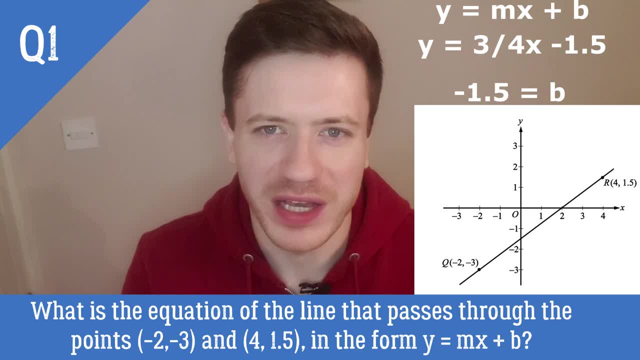 it crosses over the y-axis at minus 1.5. but you now have the perfect method for working out, even if they don't give it to you visually, which is most likely what they're going to do. they're not going to give you the graph, so you have to work out the plus b. how do you work out the plus b? 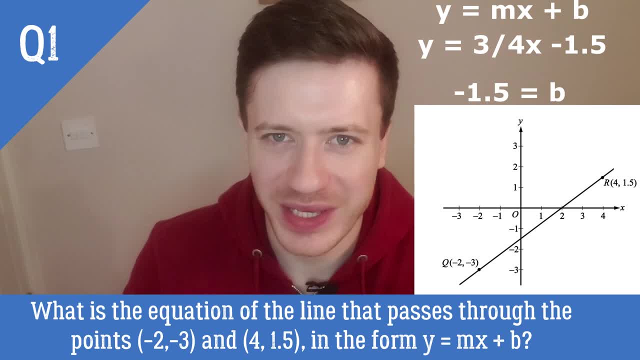 you insert one of the coordinates into the equation. after having worked out the slope, can you remember that we now have our full equation? the full equation of that line y equals three quarters x minus 1.5 or minus three over two. same thing. i've seen some students make the mistake of writing. 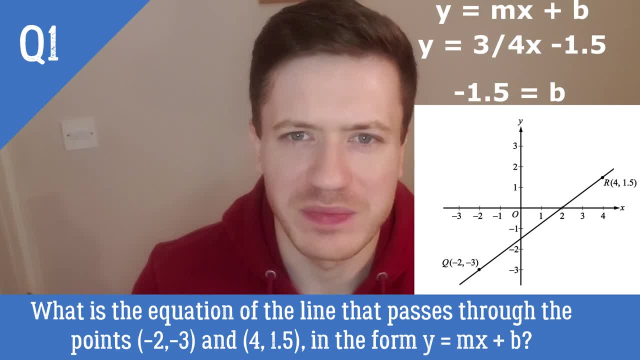 something like y equals three quarters times minus two plus whatever. but no, we only use one of those coordinates just to work out the m and just to work out the plus b. we don't actually use those coordinates in the final equation. we just work out the m and just to work out the plus b. 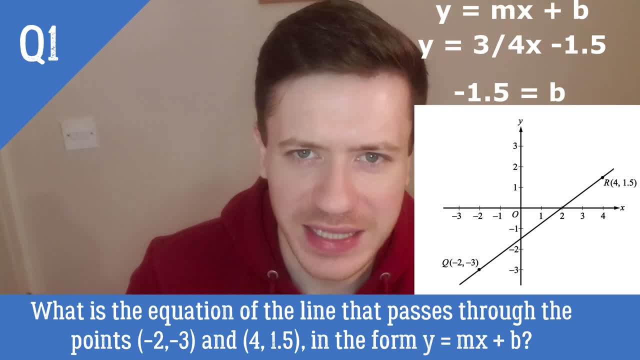 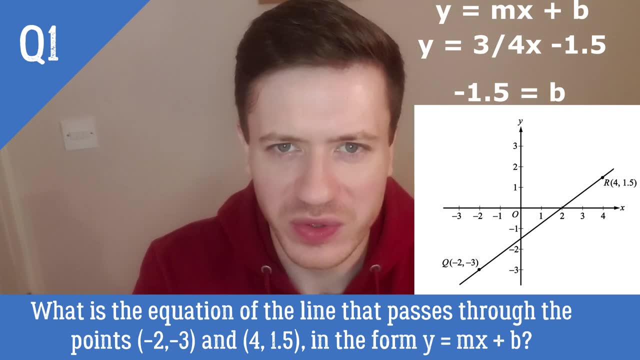 so we're going to use the m and just to work out the m and just to work out the plus b. the final equation just simply has the m and the b written with x and y untouched. y equals three quarters x minus 1.5. that is the equation of the line at the end we're going to. 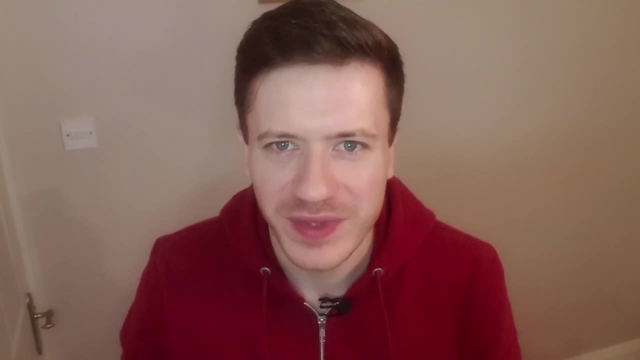 do an example that brings this all together for a final time. so don't worry if you think you need a bit more practice, but for now i'm going to move on to our next topic, which is writing out that equation in the form a, x plus b, y plus c, equals zero, which is how you'll sometimes see it, believe. 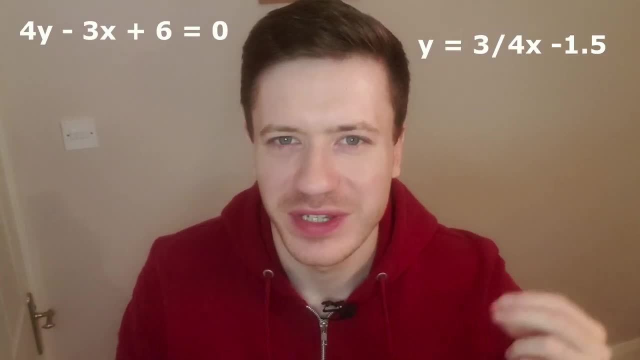 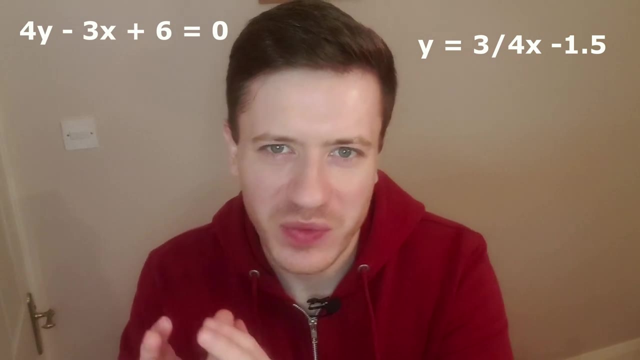 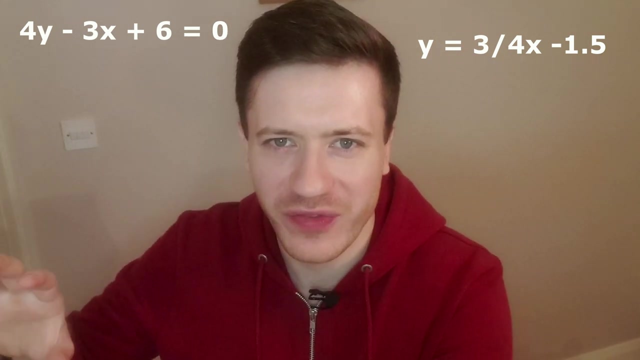 it or not, the line we just worked out is equal to four. y minus three. x plus six equals zero. how so? well, we've simply moved it all to one side, keeping a zero on the right, and then multiplied everything by four to get rid of both fractions. why do we do this? 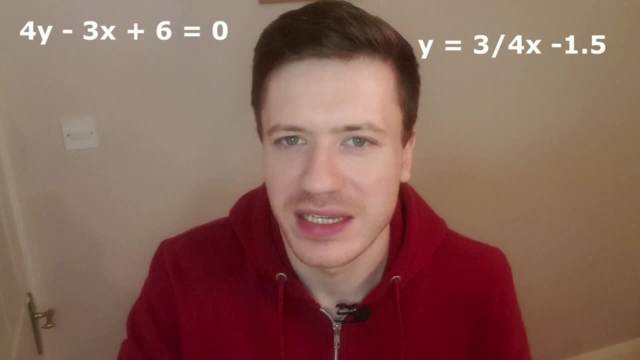 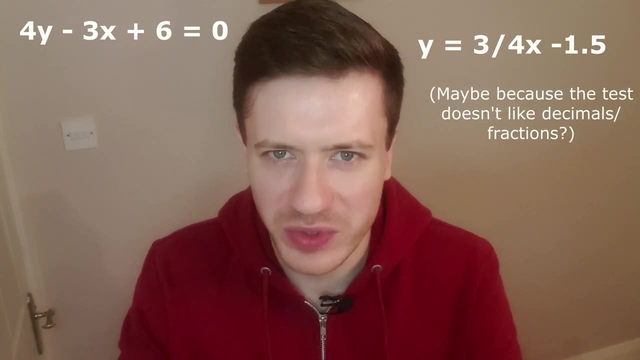 simply because for some people that's an easier way to write it and, more specifically, sometimes the gmat or gre would prefer you write the equation like this. so it's good to know what to do. you've done the hard work. you've done the coordinate geometry. this is just basic algebra. 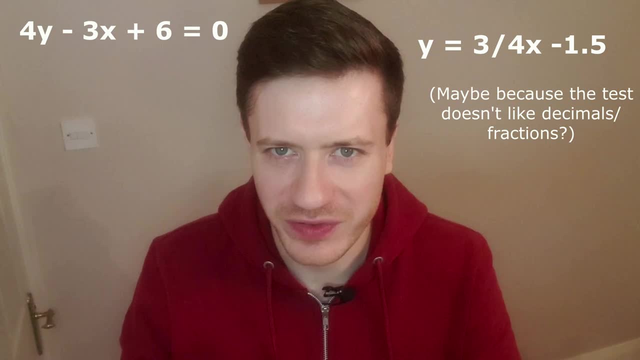 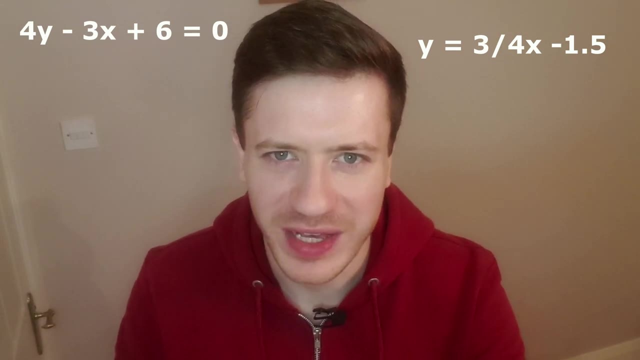 move everything to one side and always multiply to get rid of fractions, so that equation that we worked out, y equals three quarters x minus 1.5 is identical to four. y minus 3x plus six equals zero. now i've got one final topic i want to cover before i. 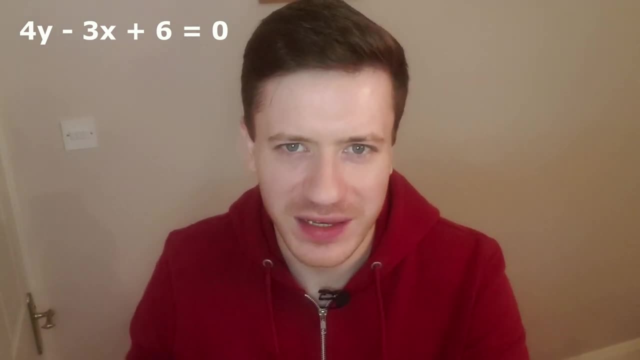 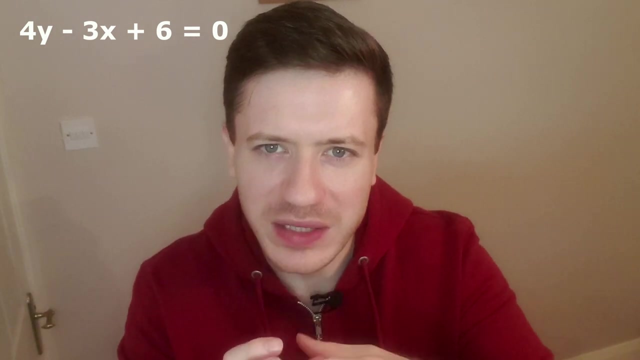 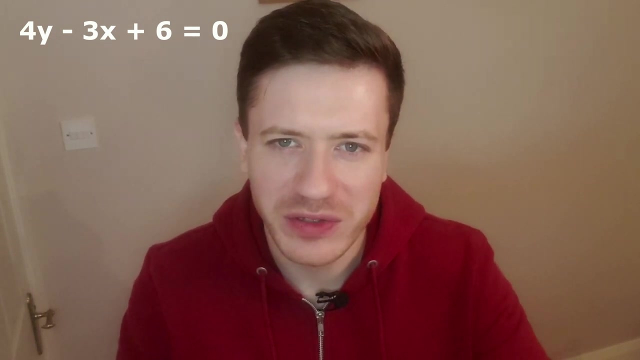 move on to parallel and perpendicular lines, which is the last topic of this video, and that is: how do you find the x-intercept? we've talked about finding the y-intercept of a line by putting the coordinates in and then working out the plus b, but how do you find the x-intercept? so the x-intercept? is where the line crosses the x and the y beat back all the zeros. it's actually called Hamilton's and b and b is where the y is. So the x-intercept is where the line crosses the x and the y crack winning, so the x-intercept is where the x is. 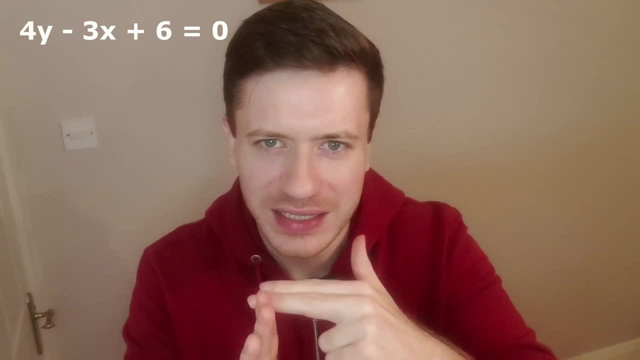 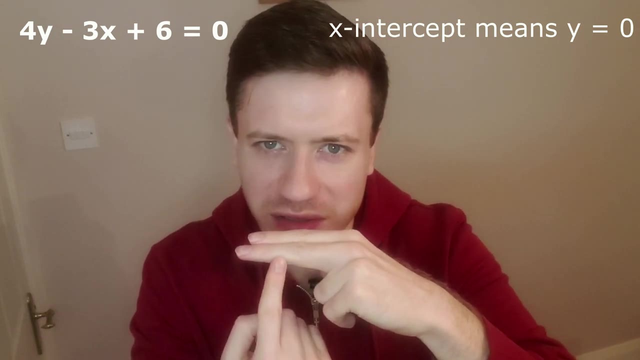 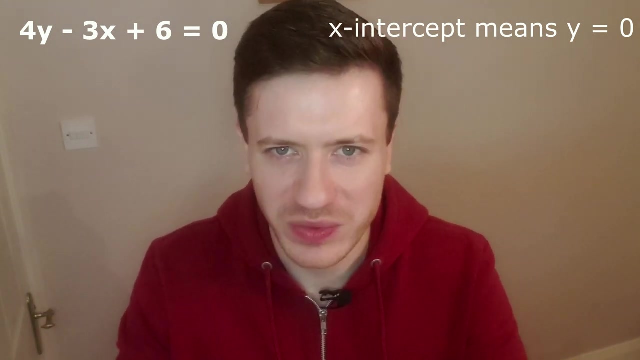 axis, And where the line crosses the x-axis, it will have a y-coordinate of 0. It won't be off the ground at all. The y, the vertical, will be 0. And that's the secret. You replace y with 0, and that will give you your x-coordinate, That will give you your x-intercept. Let's 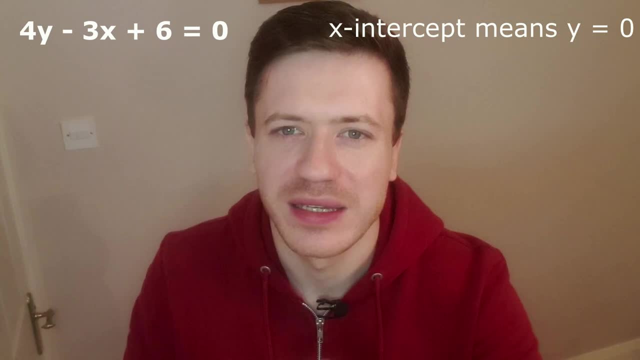 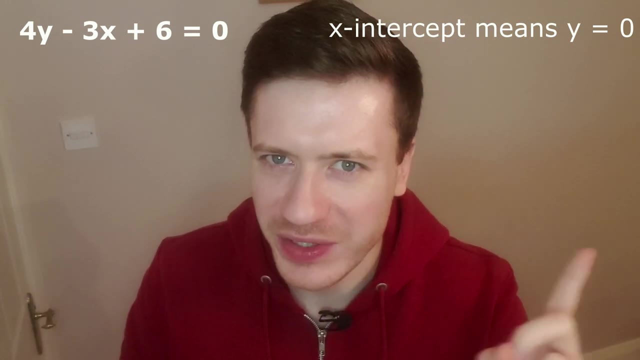 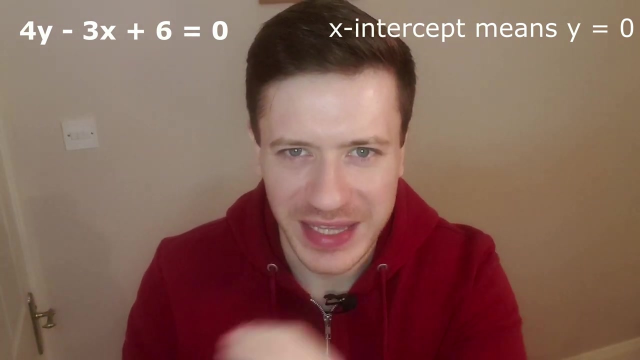 quickly do that with this line that we have here: 4y minus 3x plus 6 equals 0.. Can you quickly tell me the x-intercept, And I don't want a smart answer by looking at the graph. I want you to tell me if we had no graph there, Hopefully you replace the y with a 0 to find. 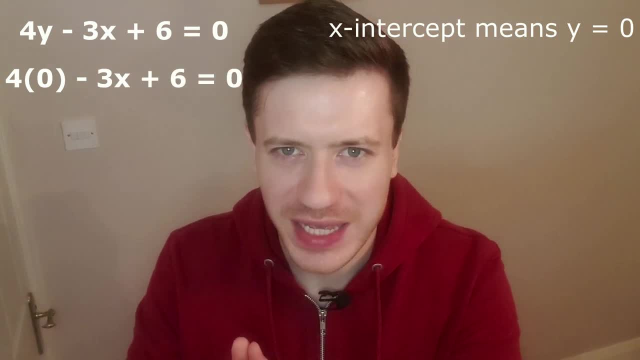 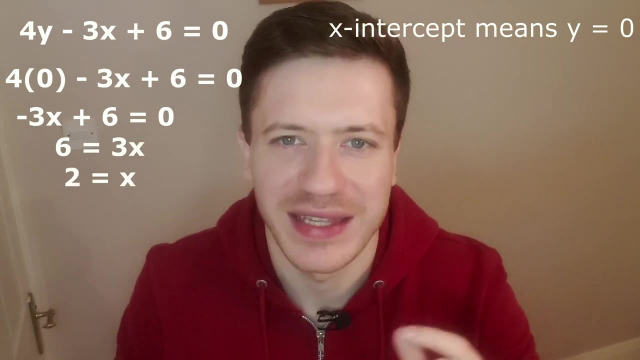 the x-intercept And you've got minus 3x plus 6 equals 0.. Adding 3x to both sides, we have 6 equals 3x And then divide by 3, 2 equals x or x equals 2.. So that's the x-intercept. 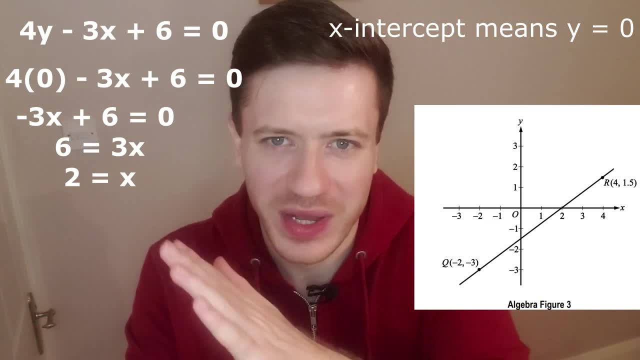 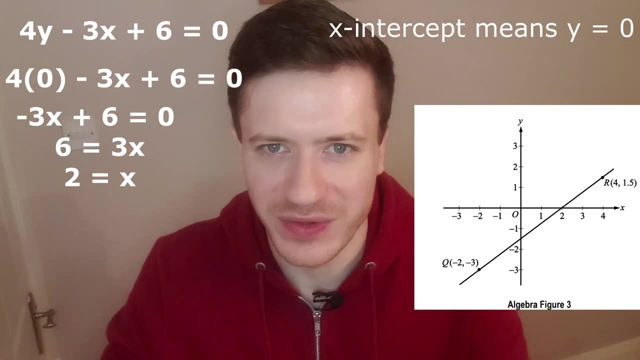 which we can confirm by looking at the graph, is indeed Where the line crosses the x-axis. at x equals 2.. Or the coordinate would be called 2, 0.. You guys are so lucky today because I'm going to be covering yet another couple of topics. 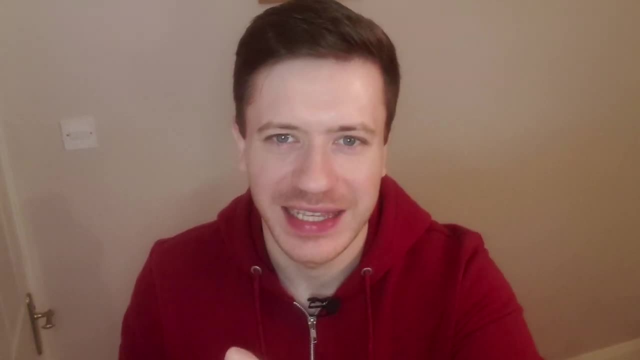 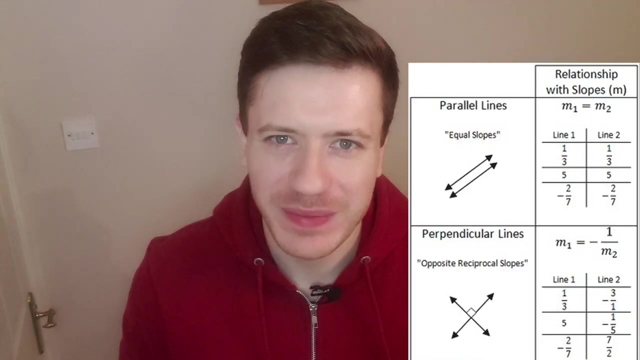 in this same video. Please hit the like and leave a comment if you've made it this far. The topic is parallel and perpendicular lines, And the diagram I have on screen just shows you what that means visually. So parallel lines have the same length, but they're not. 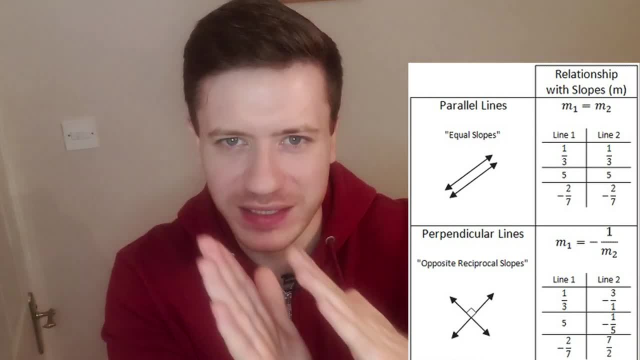 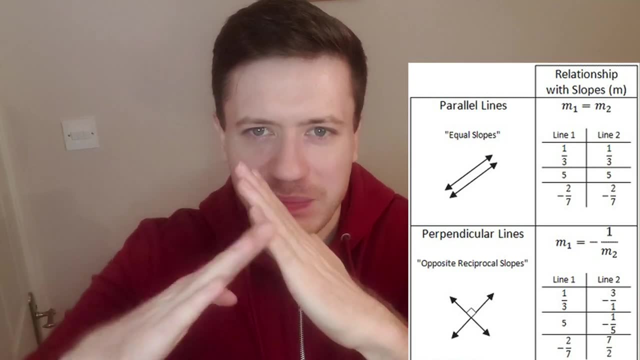 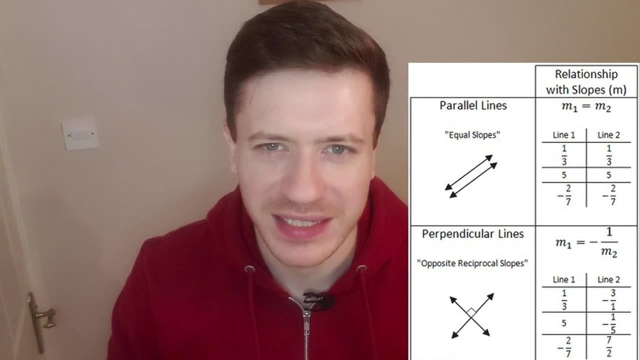 the same slope, the same gradient, and they will never meet. No matter how long they carry on, they will never touch each other. Those are parallel lines. Perpendicular lines, on the other hand, cross over exactly 90 degrees. But how will that be tested in the GRE? and 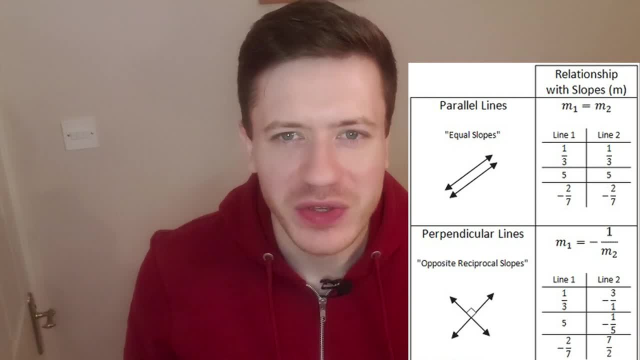 the GMAT, The parallel lines bit is a bit easier. You can tell if the equations of two different lines are parallel by checking if they have the same slope. If the m's are the same, then they have the same slope and therefore are parallel. You. 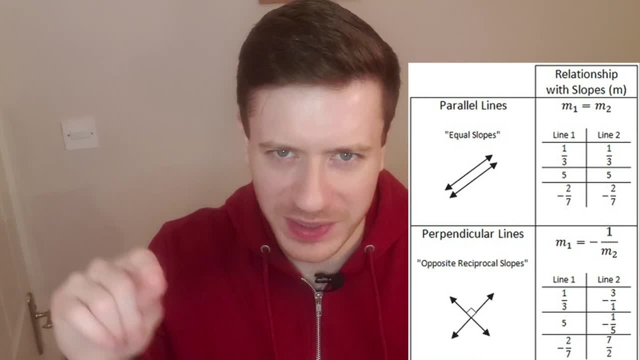 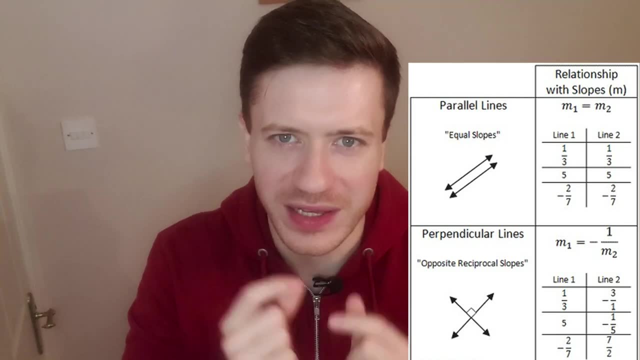 might need to rearrange the equations to put them in the form: y equals mx plus b, to see what the m's are. But if you find out that the m's are the same, then you have parallel lines. But how can we tell if the lines are perpendicular? This is the funky bit, that 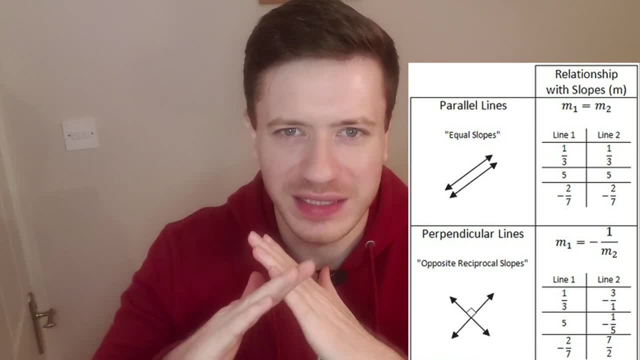 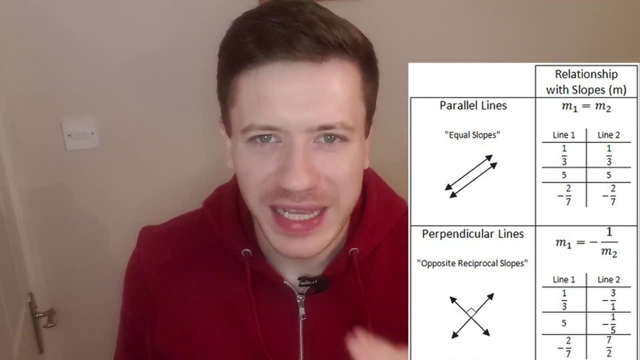 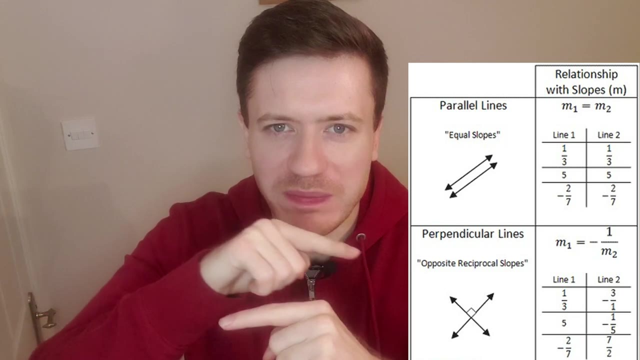 some people struggle to remember. Perpendicular lines have slopes that are the negative, reciprocal of one another. What that means is: if my line has a slope of five and your line is perpendicular, the slope of your line will be the negative of that. so that's negative. 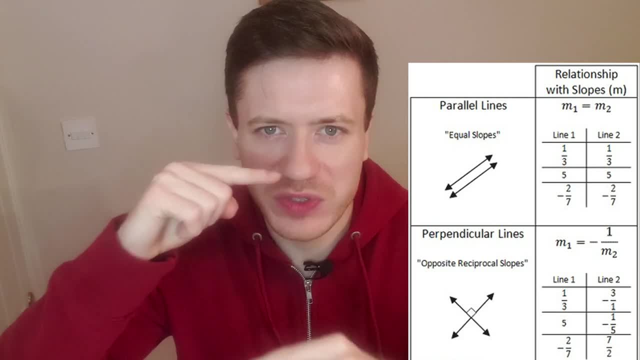 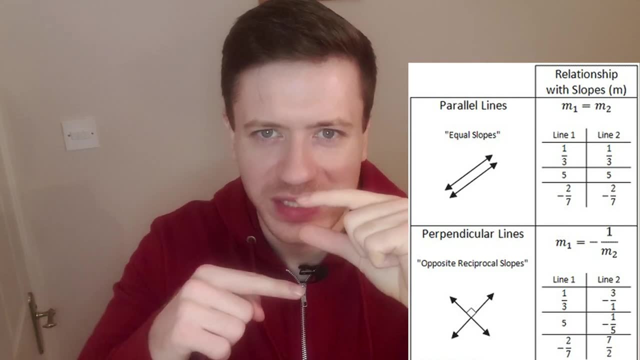 five, but also reciprocal. Reciprocal just means flipping a fraction And you might say five isn't a fraction, but five is five over one. So if we do the reciprocal of that, we get one over five. Bringing those two things together, if my slope is five, your slope is five. 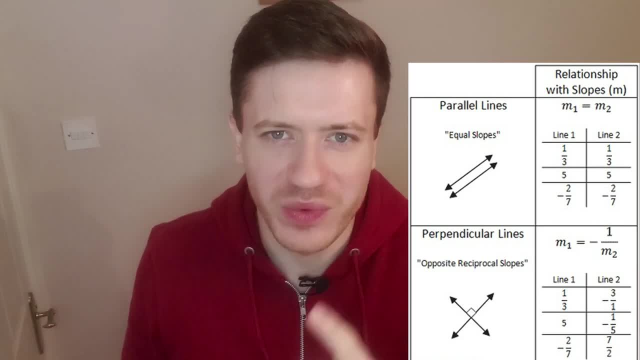 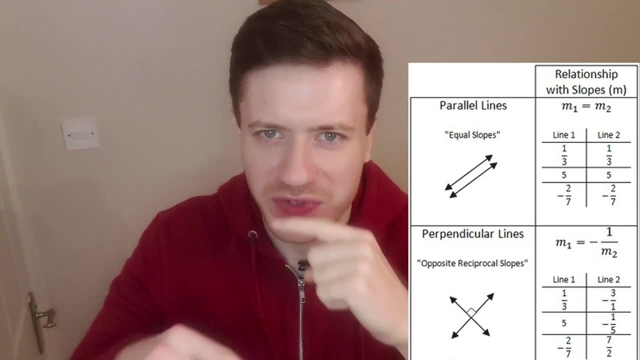 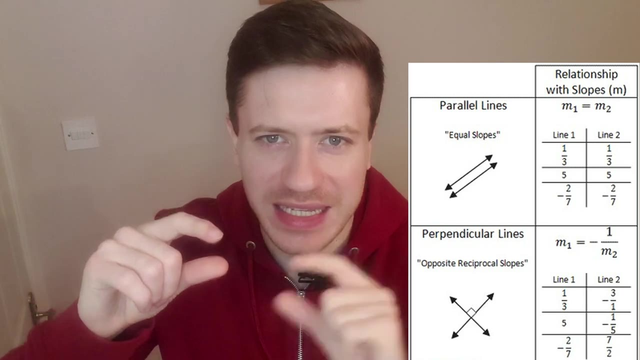 Your slope as a perpendicular line would be negative one over five. If my slope is a third, your slope is the negative reciprocal of that. The reciprocal of a third is three over one, which is three, and the negative makes it negative three. And that's how you deal with. 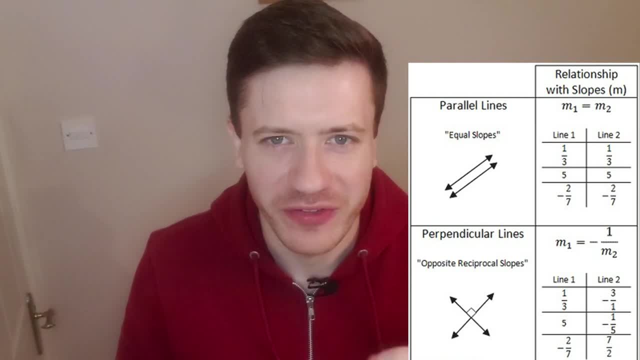 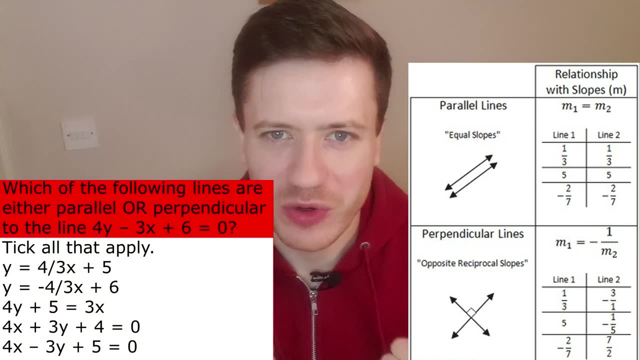 perpendicular slopes. I'm going to bring that together in the following GRE style question: Which of the following lines are either parallel or perpendicular to the line with the equation: four, y minus three, x plus six equals zero? Before you get started, you might have realized that you're going to have to. 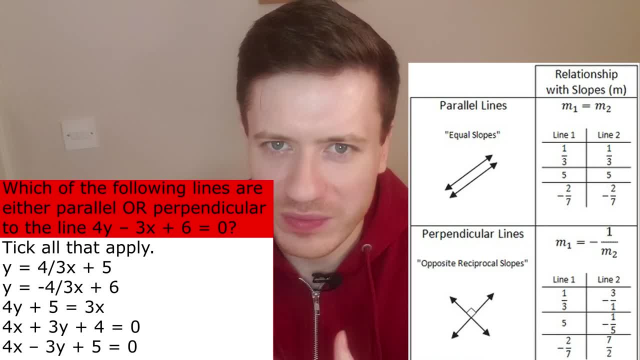 rearrange each of these equations, if they're not already in that form, into the form: y equals mx plus b. Once you've done that, look at the m's, and if they're the same, it means they're parallel to our original line, And if they're not, it means they're parallel to our original line. 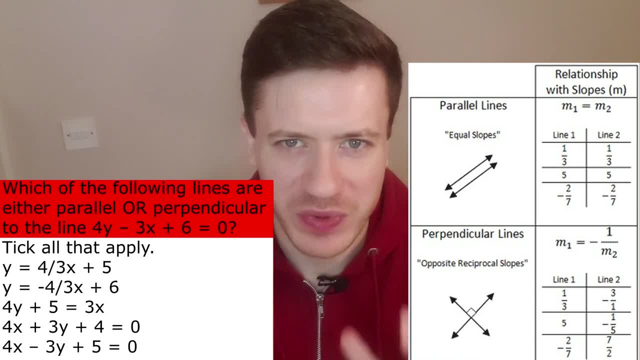 If they're the negative reciprocal, they are perpendicular. So pause the video, have a go yourself. If you can't do it, I'm now going to explain. Many of you might have been thinking: well, what is the slope of that line? four y minus three, x plus six equals zero. Well, we did do this. 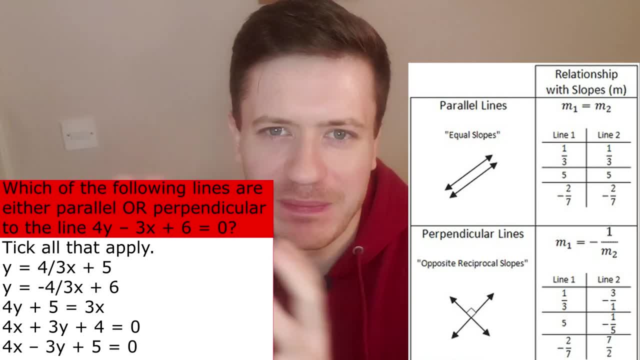 earlier. but what you're going to have to do is rearrange it back into the form it was before, with just a single y equals blah, blah, blah, x plus blah, blah, blah. So rearranging that, we push the minus three, x and we're going to have a slope of four y minus three, x plus zero. 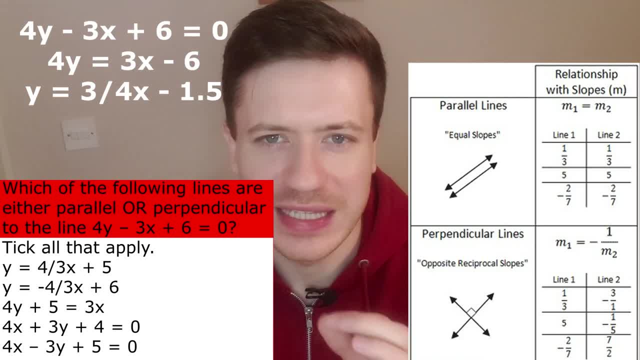 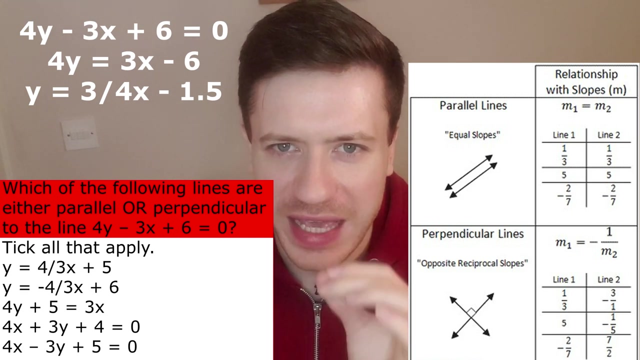 And the plus six to the other side. So we have four. y equals three x minus six. And then we divide by four, So y equals three quarters x minus 1.5, back to where we were before, with our slope being three quarters. Your job is to rearrange all the others in that same form And look at the m's. 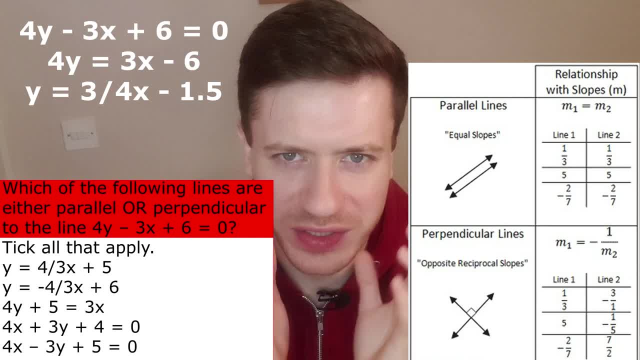 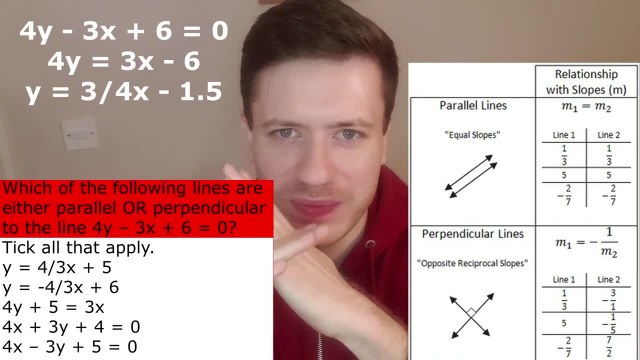 look at the numbers next to x. Those are our slopes, And if they're the same as three quarters, that means we found a parallel line. If they're the negative reciprocal, we found a perpendicular line. Just quickly. what's the negative reciprocal of? 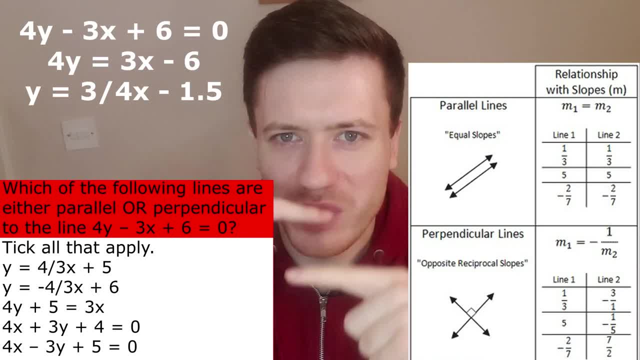 three quarters, It would be four over three with a minus. So minus four over three. That's what you're looking out for. to find a perpendicular line. I'm not going to go through all of them, but you should have found that the second line was perpendicular to our original line. 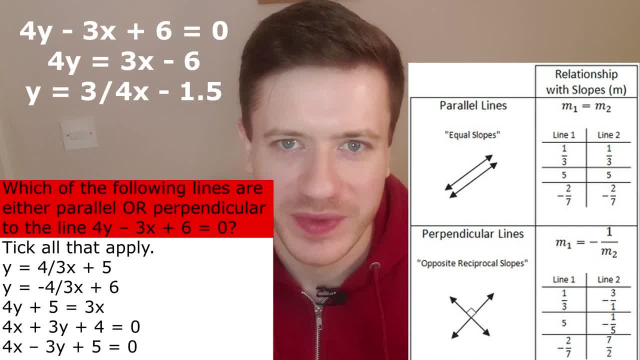 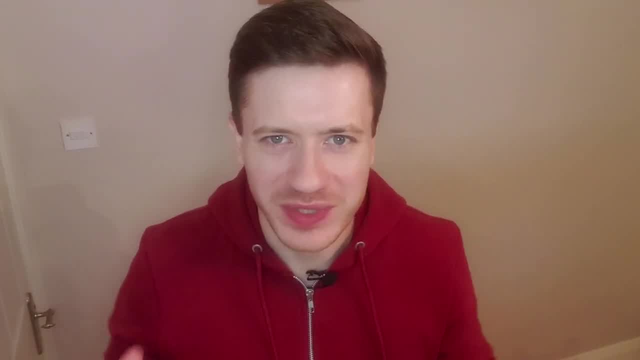 And the fourth line was perpendicular And the first and fifth were neither parallel nor perpendicular. I said that there will be a question at the end that brings it all together, And here it is. In fact, it's a multi-part question, testing many different things, So I just thought it'd be. 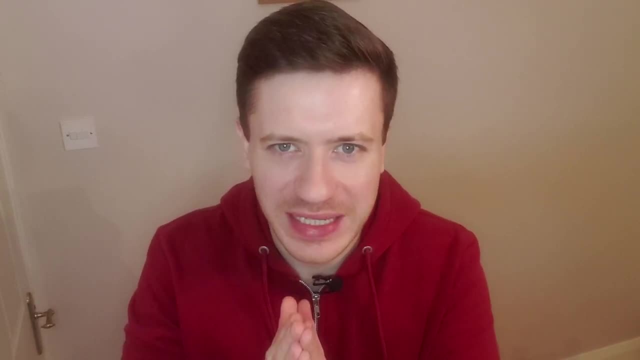 worth doing to cover all the different knowledge you might need to know. for at least 80% of the questions that you'll see on coordinate geometry in the GMAT and GRE, You can see the question on screen And you can see that the question on the GMAT and GRE are both perpendicular, So you can. 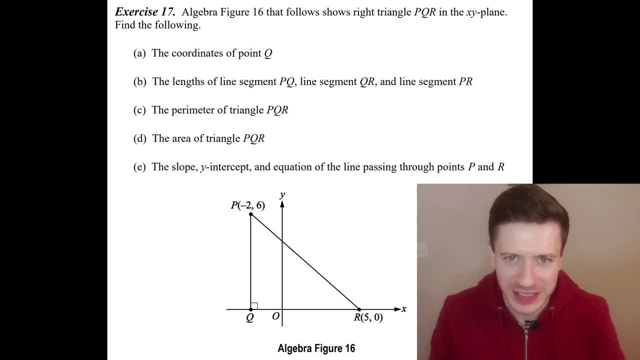 where we have a line and then a vertical line going down from one coordinate. And the first question, question A, is to work out the coordinates of point Q, which is vertically beneath point P. It's a nice little warm-up to get us started, As with all of these questions, 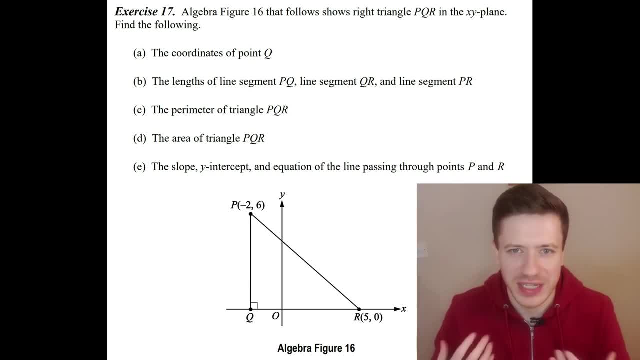 feel free to pause the video, work them out yourself first, or you can just listen to my explanation. So point Q is vertically beneath point P, which means it's going to have the same x-coordinate. The horizontal direction of both coordinates is the same, So the x-coordinate is: 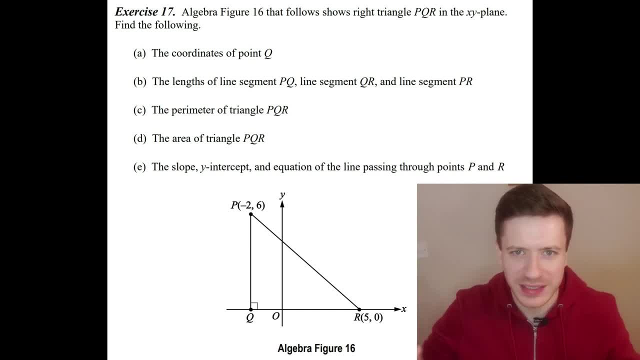 going to be minus 2, and because it's on the x-axis, the y-coordinate is 0.. That's our first question answered. The coordinates of point Q are minus 2,, 0.. For B, they want the length of each of the line segments. Now, two of those are easy and the third one involves a topic. 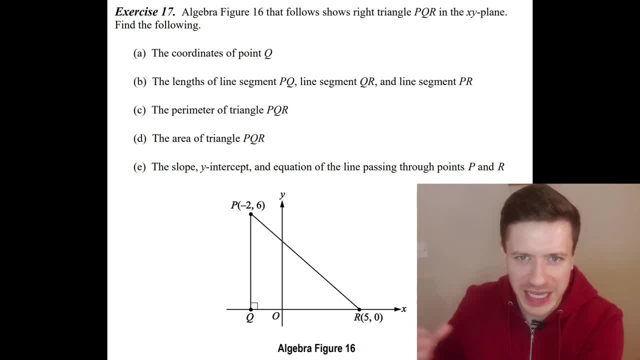 I did in an earlier video that I would strongly recommend you check out if you don't know about it. So the length of the line segment PQ is simply 6. It doesn't move at all horizontally, it just goes up 6. So that's a length of 6.. The length across from Q to R goes from minus 2 up to 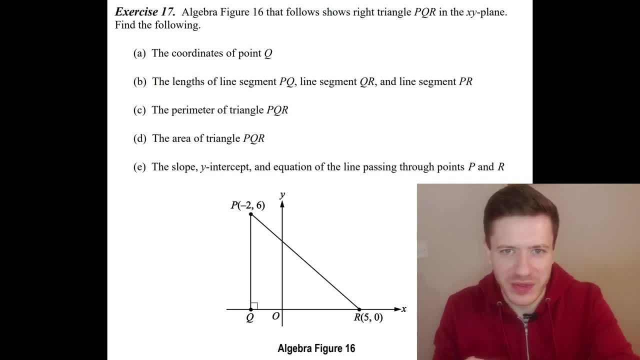 5,, and that's a length of 7.. How to work out the line between P and R? Well, I've done another video on the distance between two coordinates, so I strongly recommend you check that out. But for now, briefly, we're just 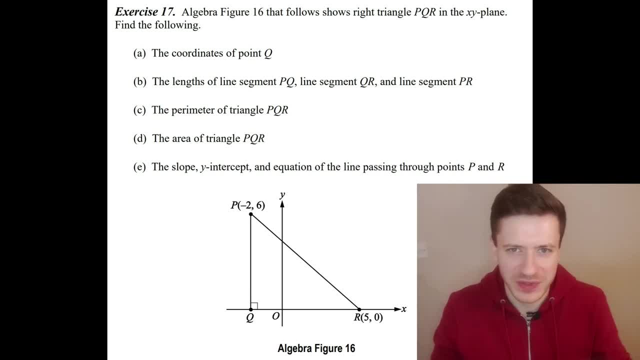 going to do Pythagoras. We're just going to do 6 squared plus 7 squared and then square root. the answer: 6 squared is 36,, 7 squared is 49.. Adding those two up, I believe we have 85, and the square. 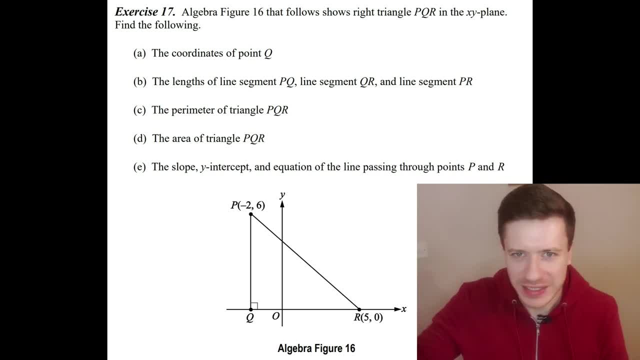 root of that you can do on a calculator, but you could just write root 85, or in the GRE, if they wanted a decimal, you could type 85 and then press square root and it should be something like 9.1. 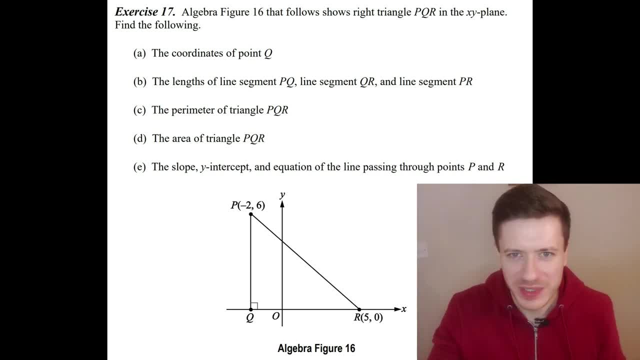 or 9.2.. Question C is easier. The perimeter: you just add up 6,, 7, and the 9.2, and that's your perimeter. That's fine. Likewise, the area shouldn't cause you any problems. That's just the base of 7. 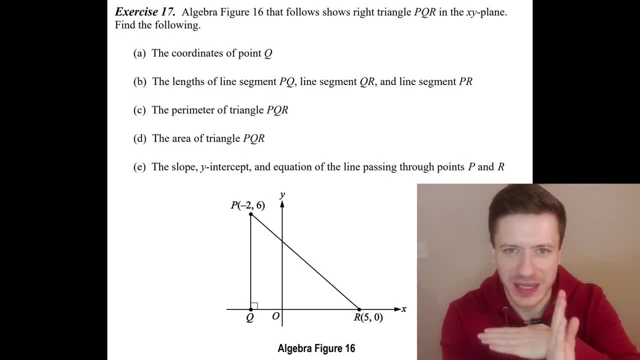 times the height of 6, divide by 2.. 7 times 6, divide by 2.. I believe 21.. It's the part E that I want to cover, because that covers what we've done in the earlier part of this video. What is the slope y-intercept and the equation of the line going? 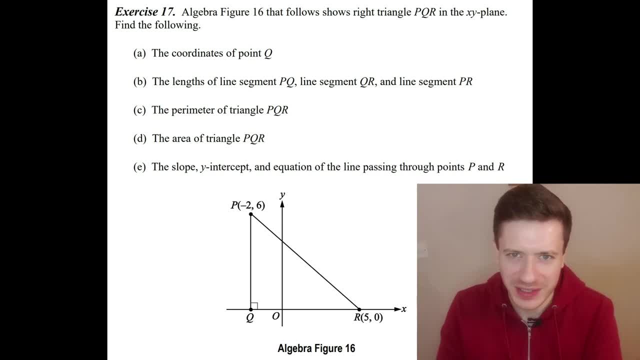 between P and R. Let's take each of those in turn. For the slope, I'm going to use the rise over run approach. How far have we risen to go? from minus 2, 6 to 5, 0? Focusing on those y-coordinates of 6 and 0.. Well, we have fallen actually by 6. We haven't risen by. 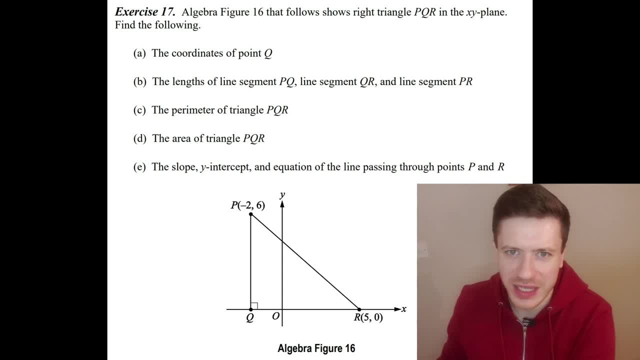 6.. To go from the coordinate on the left to the coordinate on the right, we have actually fallen by 6.. So our rise is minus 6.. What's our run? to get from minus 2 all the way to 5? Our run if we? 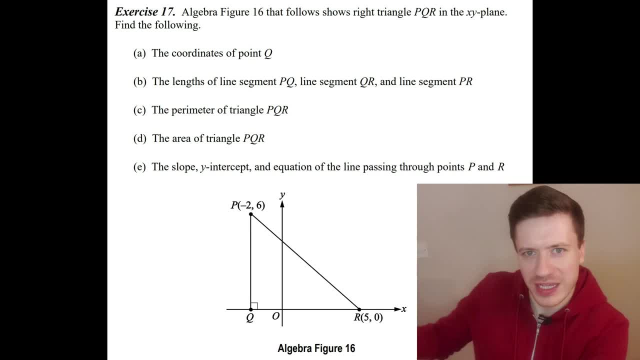 look at the x-coordinates- is 7, because we've gone in the right by 7.. So our rise over run is minus 6 over 7.. That is our slope. Do you remember how to find the y-intercept of the? 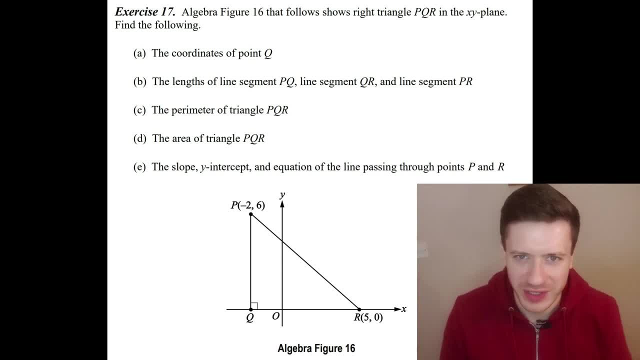 equation of a line. if it's not obvious visually from the graph, Massive brownie points to you. if you said, you write out the y equals mx plus b and then insert one of the coordinates, The equation so far is: y equals minus 6 over 7x plus b. and we don't know that plus b, And we're going. 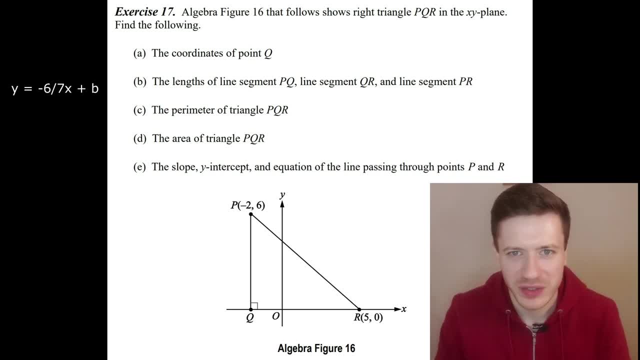 to work it out By replacing the x and the y with one of the coordinates. Let's do 5 and 0, the coordinate on the right. It doesn't matter which coordinate we use, but that one looks easier. Replacing the x. 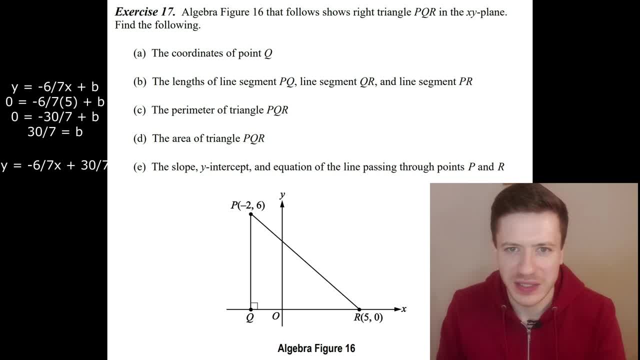 with a 5 and the y with a 0, we have 0 equals minus 6 over 7 times 5 plus b. Minus 6 over 7 times 5 is minus 30 over 7 plus b, And pushing that minus 30 over 7 to the other side would give.